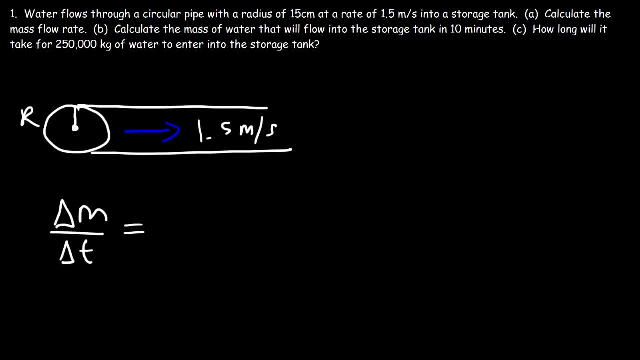 the change in time. Mass is density times volume, because density is mass divided by volume. So if we multiply both sides by v, we can see that m is density times volume. So the density times the change in volume is equal to the change in mass. Now, volume is the amount of mass that 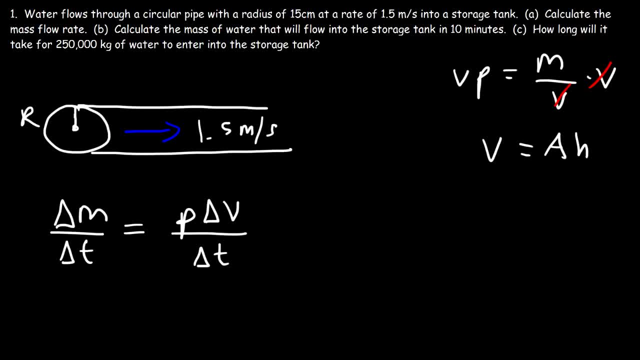 flows through the pipe. So we can multiply both sides by v. So we can say that volume is area times height. So in this case, since we're dealing with a vertical displacement, we can say that the volume of a cylinder, a horizontal cylinder, is the cross-sectional area times the vertical displacement, So we can say a. 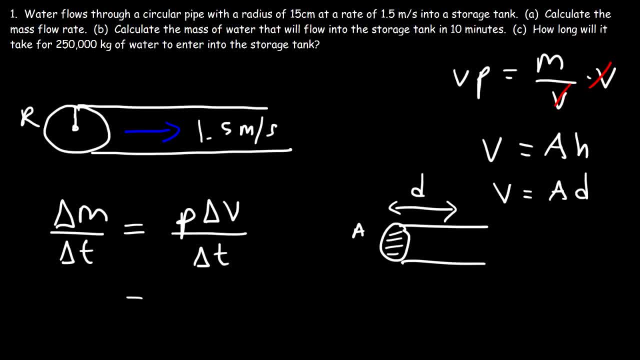 times d instead of a times h. So the change in volume is going to be the area times the displacement, which we'll call delta D. The area doesn't change in this problem, so I didn't put a triangle next to the A. 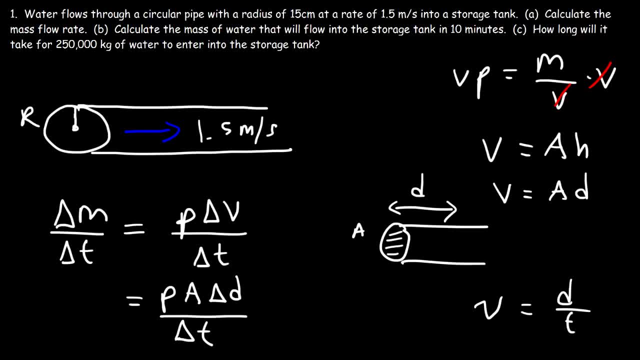 Now, velocity is displacement divided by time, So we can replace D over T with velocity. So therefore this will give us the mass flow rate equation. So the mass flow rate is equal to the density of the fluid, times the cross-sectional area times the speed of the fluid. 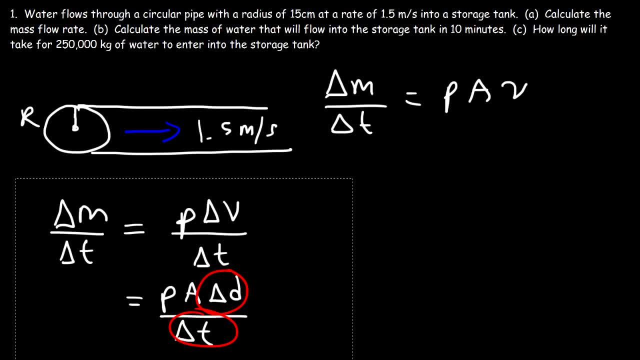 how fast it's moving. Now we have the density of water. At least you should know it. The density of water is 1,000 kilograms per cubic meter. Now the cross-sectional area, or the area of a circle. 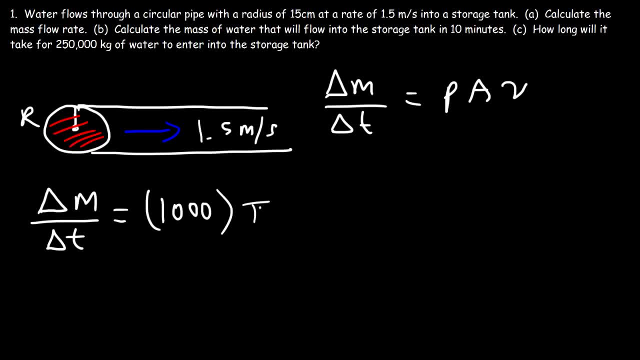 is pi? r squared. Now, the radius is 15 centimeters and we've got to convert that to meters. so we can do so by dividing 15 by 100.. So that's 0.15 meters, and don't forget to square it. 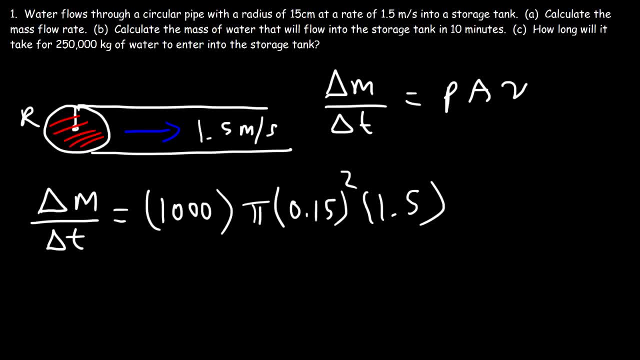 And then let's multiply it by the speed of the fluid in that pipe, So it's going to be 100.. I mean it's going to be 100.. So it's going to be 100.. 1,000, rather times pi, times 0.15 squared. 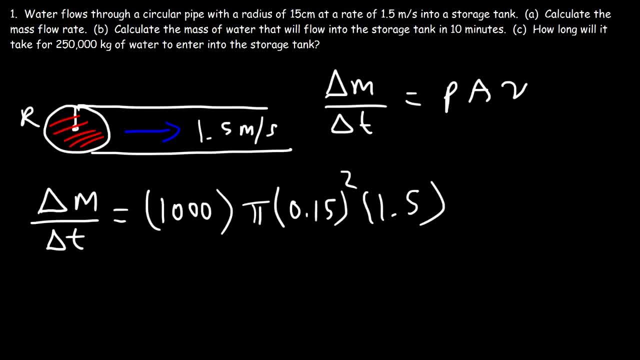 multiplied by 0.5.. So the mass flow rate in this problem is 106 kilograms per second. Now let's move on to Part B. Part B: Calculate the mass of water that will flow into the storage tank in 10 minutes. 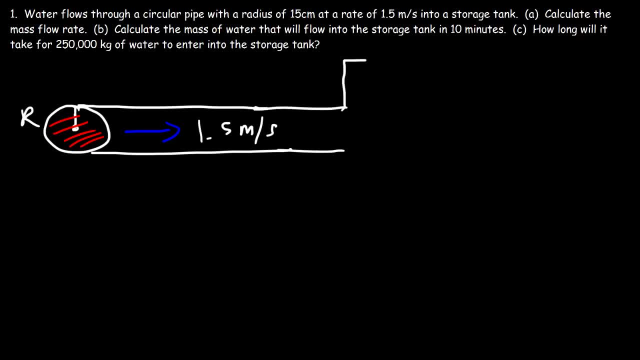 So let's connect this pipe to a storage tank. Let's say water flows into the storage tank. How can we calculate the mass of water that will flow in 10 minutes? Now keep in mind the mass flow rate is 106 kilograms per second. 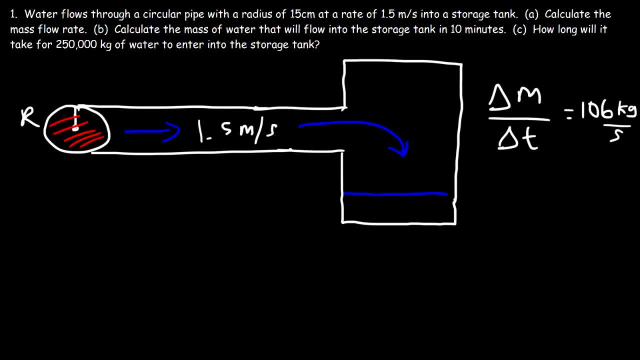 We can get the answer through a conversion process. So let's start with the time: 10 minutes. If you want to find the change in mass, simply multiply the mass flow rate by the change in time. So these will cancel. So I'm going to start with the time, which is 10 minutes. 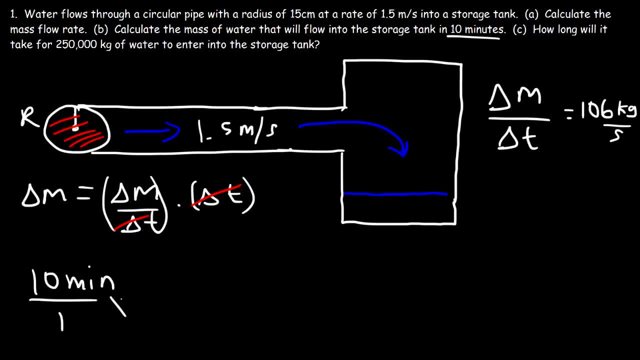 And then I'm going to convert that to seconds. Each minute contains 60 seconds, So now I have the time in seconds, which is 600 seconds. All I need to do is multiply that by the mass flow rate and that's going to give me the change in mass in 10 minutes. 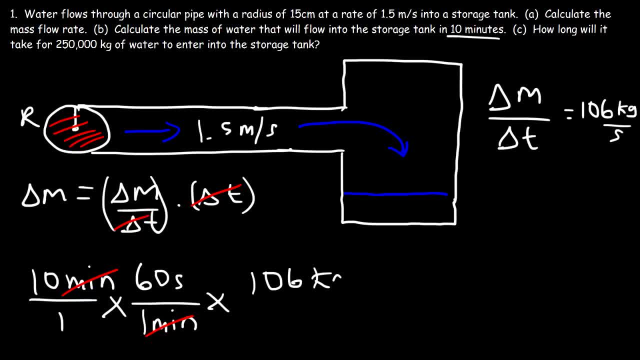 So the mass flow rate is 106 kilograms per second, And so, multiplying the time of 600 seconds by the mass flow rate of 106 kilograms per second, that's going to give you the change in time, which is the change in mass of 63,600 kilograms. 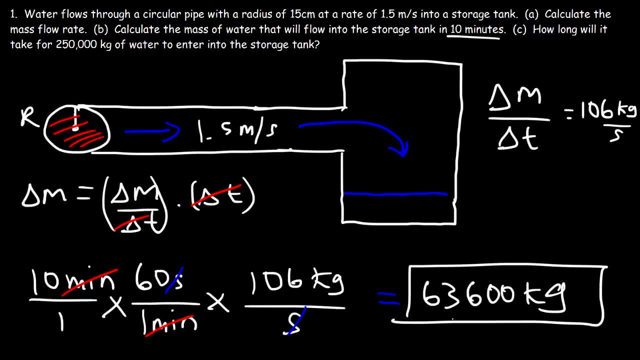 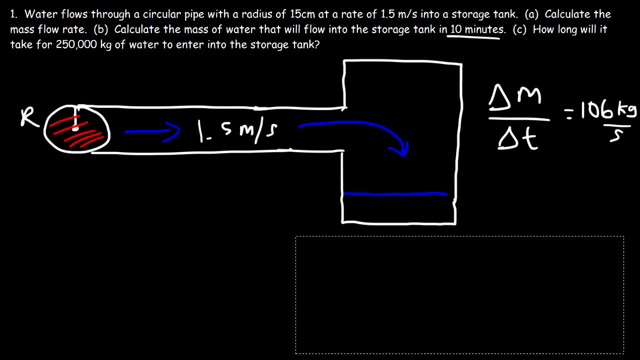 So that's how much water is going to flow into the tank in 10 minutes. Now let's move on to part C. How long will it take for 250,000 kilograms of water to enter into the storage tank? So we're looking for the time. 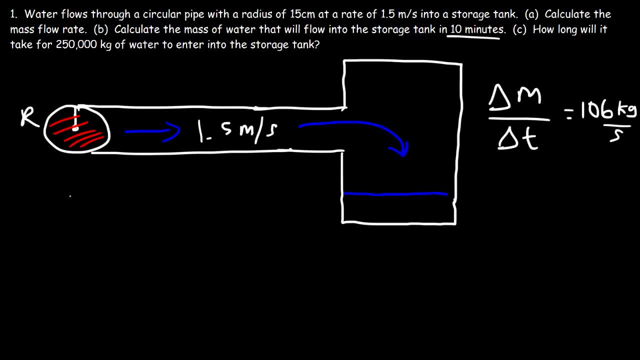 And we saw that the change in mass was equal to the mass flow rate times the time. So if you want to find the time, you need to take the mass and divide it by the mass flow rate. So let's do this using a conversion process. 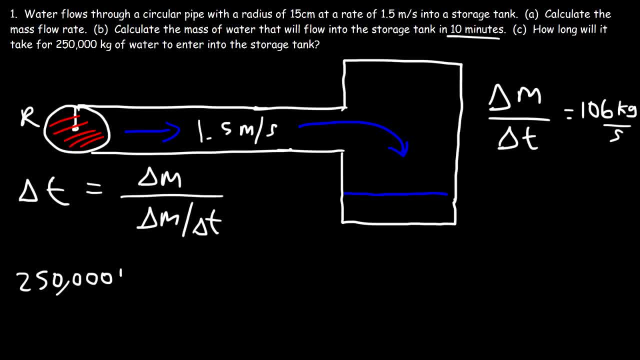 Let's start with the mass, which is 250,000 kilograms, And then let's divide it by the mass flow rate, So I'm going to put the 106 on the bottom. So 106 kilograms of water flows through the pipe every second. 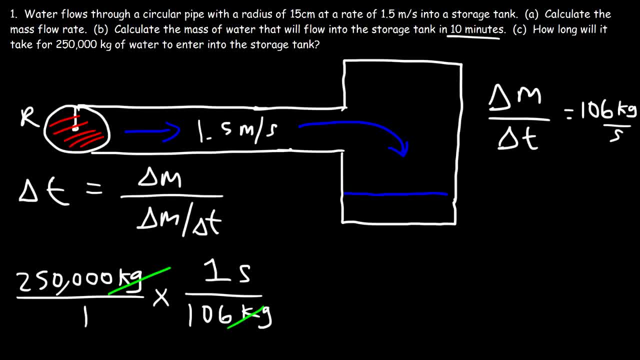 So notice that the unit kilograms cancel. and now I have the time in seconds. But chances are this is going to be a big number, so I'm going to get the time in minutes. I'm going to convert it to minutes, So there's 60 seconds in a minute. 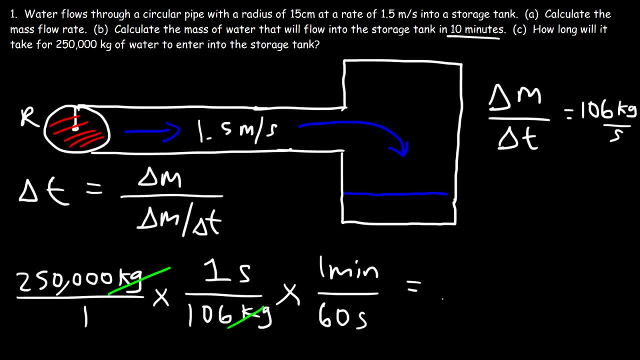 So it's going to be 250,000 divided by 106, so that's 2,358 seconds. and then divide that by 60. So this is going to be 39.3 minutes. So that's how long it's going to take. 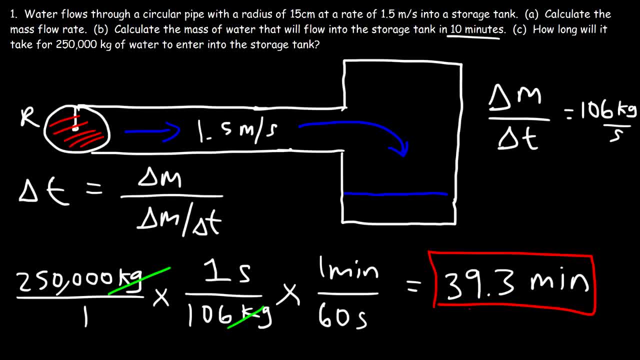 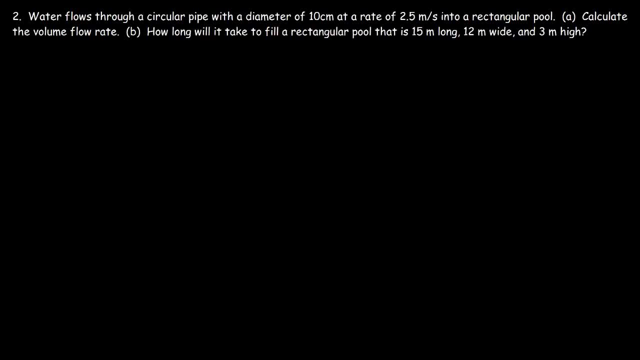 for 250,000 kilograms of water to enter into the storage tank. Now let's move on to number two. Water flows through a circular pipe with a diameter of 10 centimeters at a rate of 2.5 meters per second into a rectangular pool. 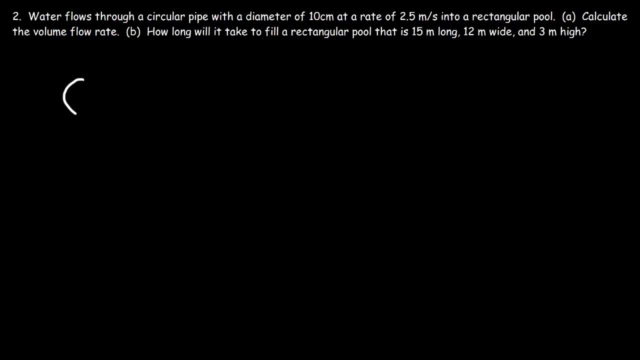 Calculate the volume flow rate. So let's say this is the circular pipe And it's flowing through it at a speed of 2.5 meters per second, And this time we're given the diameter of the circular pipe, which is 10 centimeters. 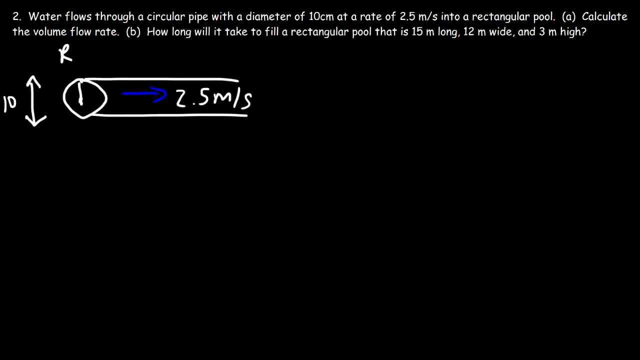 So the radius is one half of the diameter. So that means the radius has to be 5 centimeters. So how can we calculate the volume flow rate? The volume flow rate is the change in volume of the fluid divided by the change in time. 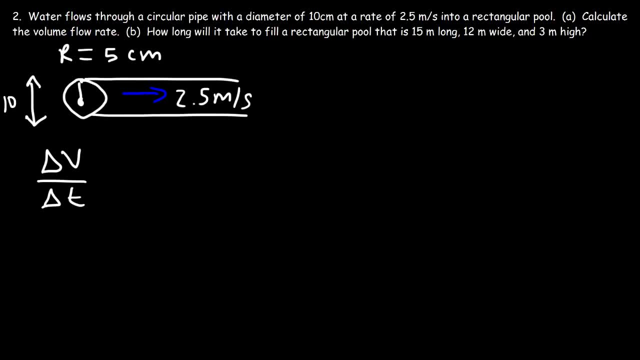 Whenever you're dealing with a rate, you're dealing with how fast something is traveling or moving. So this is how fast the volume is changing. Now volume- let me put this here- is area times height. So the change in volume is the area times the change in height. 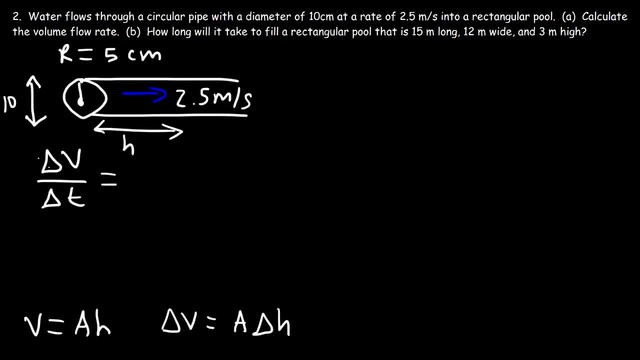 In this example only H is changing as the fluid flows. The diameter is constant, So the area is not changing. So the change in volume is A times delta H, And if we take the horizontal displacement divided by the time, that's going to give us the speed. 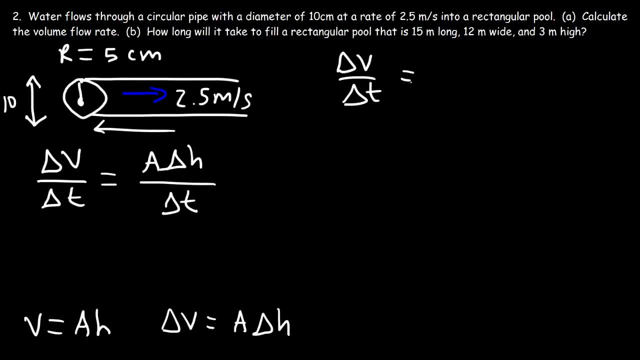 So the volume flow rate is the cross sectional area multiplied by the speed of the fluid. So let's calculate the cross sectional area. It's going to be pi r squared and then times the speed. So the radius is 5 centimeters, which is 0.05 meters. 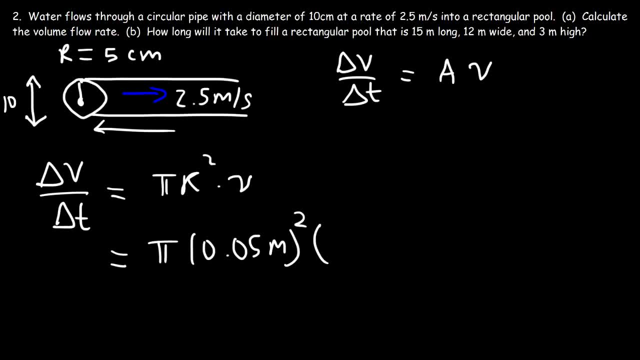 And the speed is 2.5 meters per second. So let's get the answer. So pi times 0.05, squared times 2.5, that's 0.0196 cubic meters per second. Meters squared times meters is cubic meters. 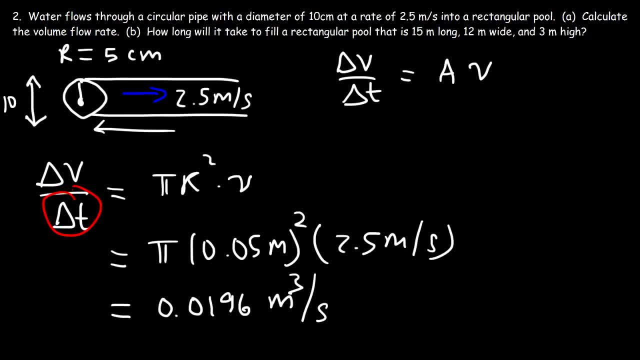 which represents the unit of volume And the unit of time is seconds. So now that we have the volume flow rate, let's find out how long it's going to take to fill a rectangular pool that is 15 meters long, 12 meters wide. 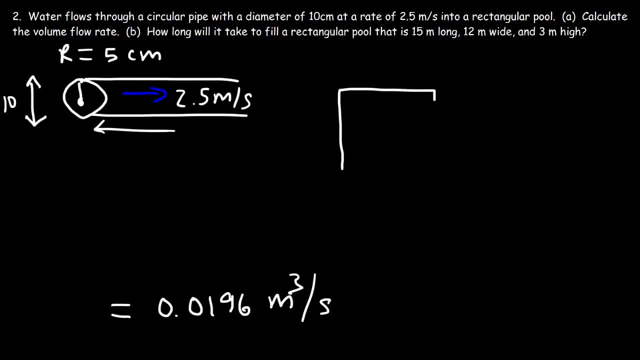 and 3 meters high. So let's draw a picture. So let's say water flows into this rectangular pool. How long will it take to fill this rectangular pool? So it's 15 meters long, 12 meters wide and 3 meters high. 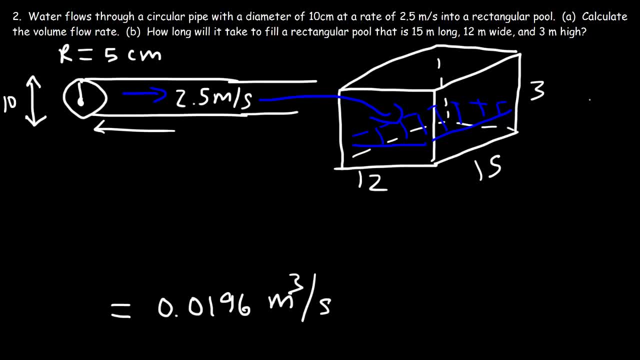 How can we find the answer? Well, we can use the conversion process, just like before. So let's start with the volume. So the volume of a rectangular prism is the length times the width times the height, So it's 15 meters long. 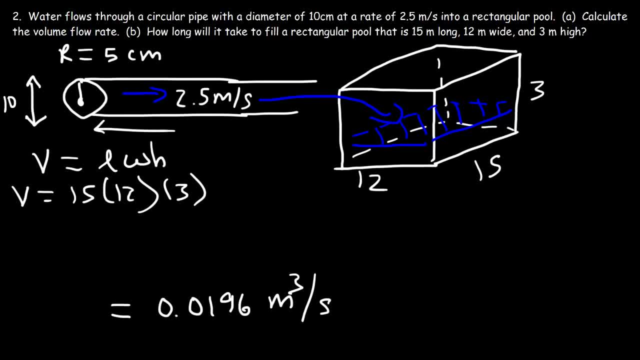 12 meters wide, 3 meters high. So 15 times 12 times 3, that's equal to a volume of 540 cubic meters. So now that we have the volume, and using the volume flow rate, we can calculate the time. 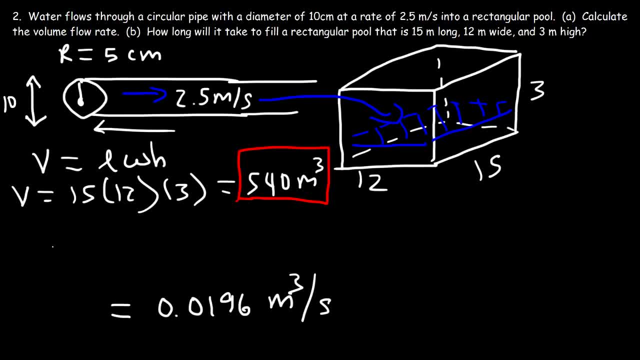 So let's start with the volume. So we have 540 cubic meters And let's divide it by the volume, flow rate, So every second .0196 cubic meters of water will flow into this pool. And now let's convert seconds into minutes. 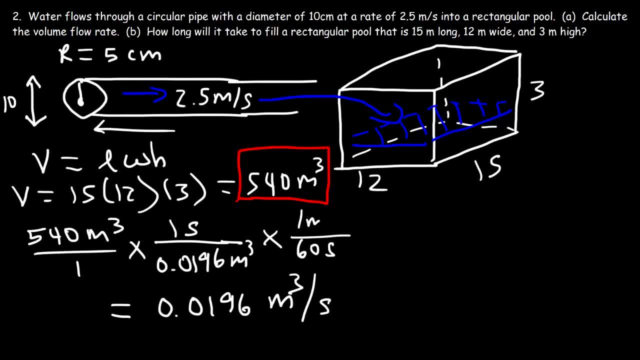 So there's 60 seconds per minute And let's convert minutes into hours, There's 60 minutes per hour. So if we take 540 and divide it by .0196,, that will give us the time in seconds, which is 27,551 seconds. 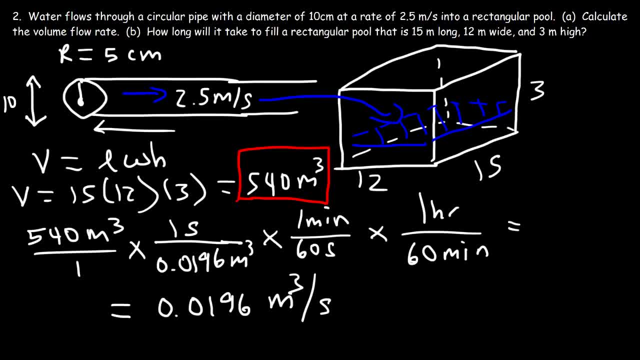 That's how long it's going to take to fill this pool. Now to convert seconds into minutes, divide by 60. So that's going to be 459 minutes, And if you divide it by 60 again, this is going to give us. 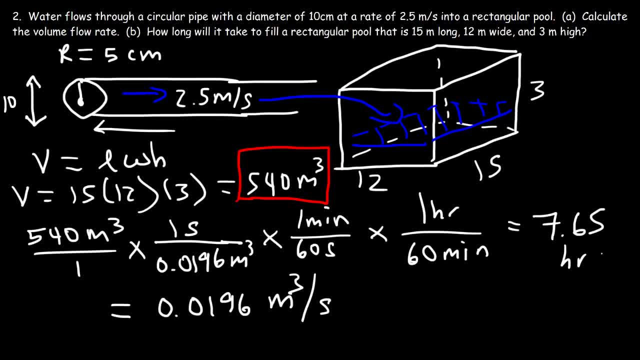 7.65 hours. So that's how long it's going to take to fill this pool when water flows through this pipe at a speed of 2.5 meters per second.